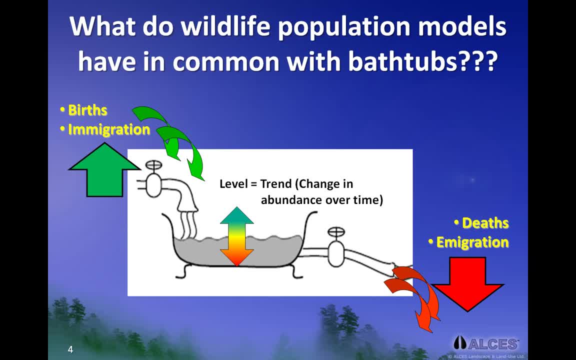 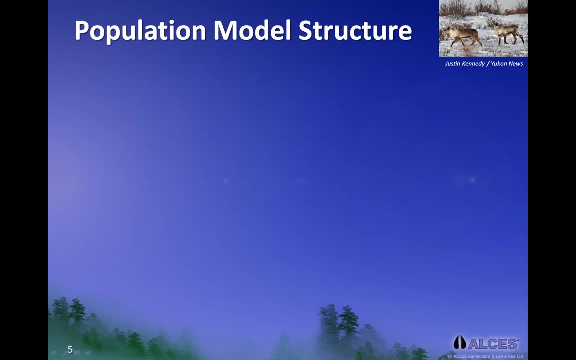 where a stock represents a group of animals and flow refers to the number of new animals added or removed. For this example, we will assume that the number of animals immigrating and emigrating cancel each other out, So let's apply the concept of a stock and flow model. 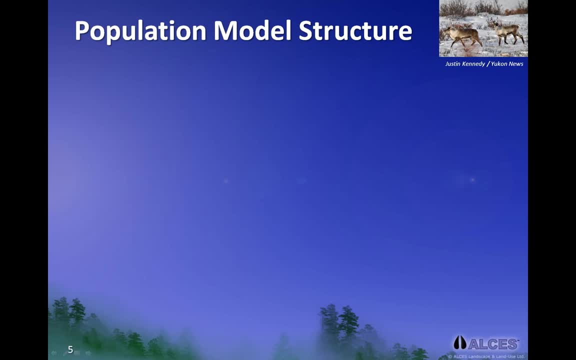 to an animal population, and we'll use caribou as an example. Firstly, we recognize that there are two sexes, female, shown above, and male, shown below, and we defined three age classes: calves, yearlings and adults. Each age and sex of caribou in this model structure represents a stock. 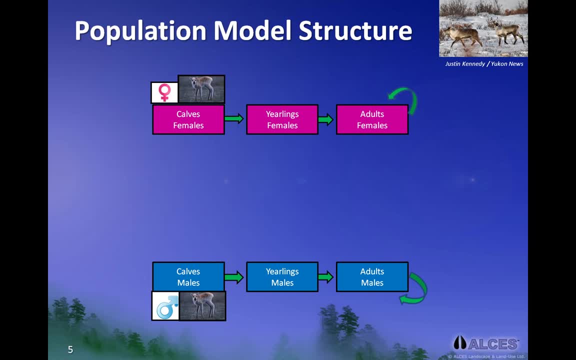 or unique group within the population. The green arrows represent inflow rates from one stock to another. For example: a certain proportion of calves become yearlings. calf survival: A certain proportion of yearlings survive to become adults. yearling recruitment. 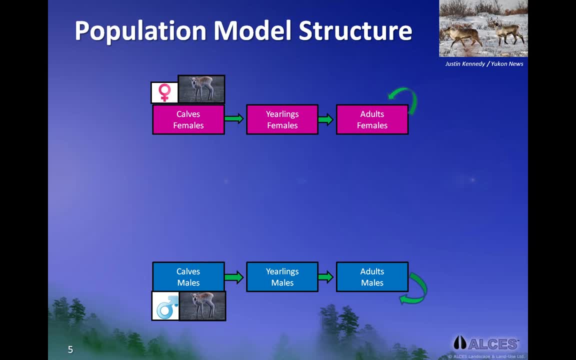 And similarly, only a proportion of adults survive from one year to the next adult survival. The long green arrow linking adult females to calves is the annual rate of births, which is generally referred to as calf productivity. Another important assumption to highlight here is that female and male calves 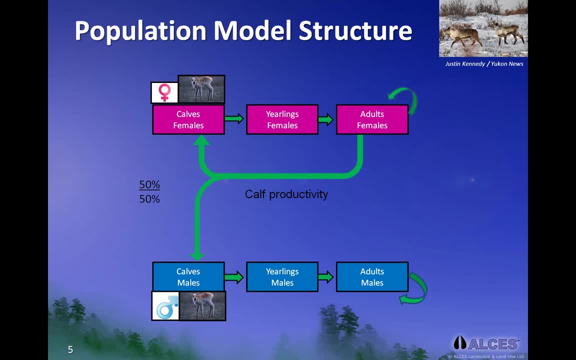 are born into the population at an even sex ratio. In contrast, the red arrows represent the number of animals leaving each of the six stocks in this stock and flow model. Simply put, the red arrows represent rates of death or mortality rates. To turn this simple conceptual model into a working model, 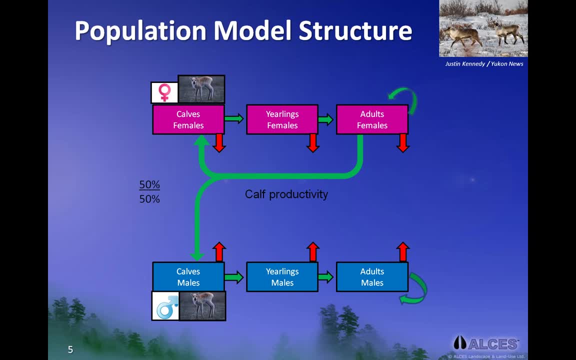 we would need to estimate the number of animals within each stock and estimate rates of birth, death and survival for each of the green and red arrows, And the final steps would be to link the stocks and flows over a defined time period, usually a year. 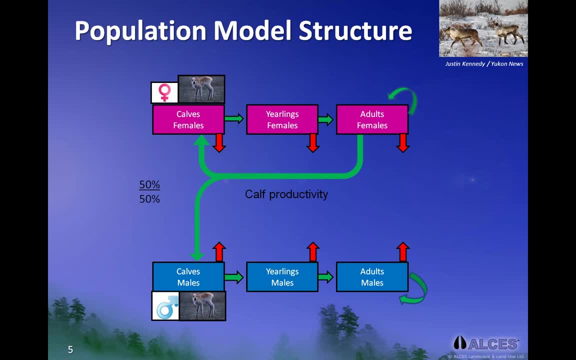 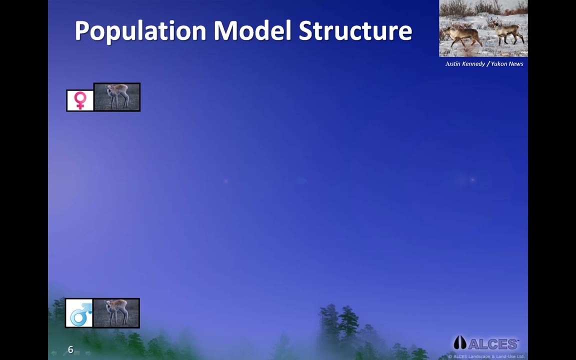 and then to write out the relationships between stocks and flows using mathematical equations. We typically need to use a computer to track and calculate all of the various equations, inputs and outputs. A simple structure can be an effective way of thinking about a wildlife population. 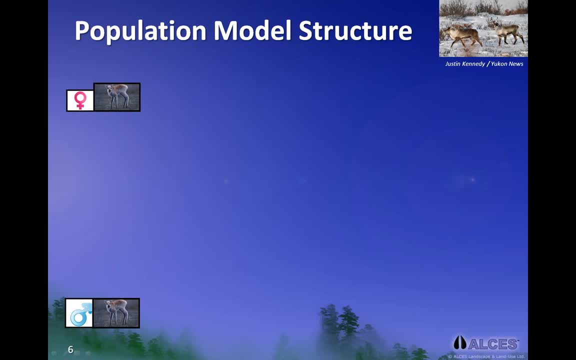 but in the real world there are many different ages of adult animals and a better model might be based upon more than one stock for adults. Here we have broken down the adult animal component into three classes: young, mature and old adults. 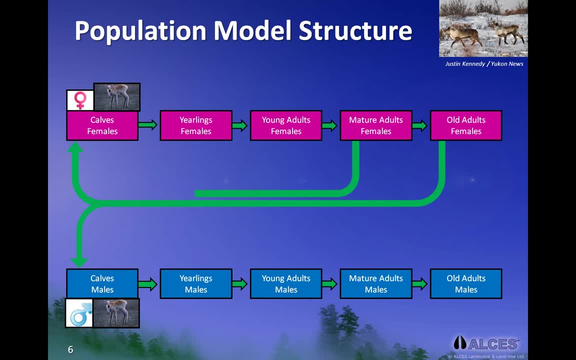 As you can see, as we add complexity and realism to models, we add the need for more detailed information, and we also have to be very clear about our assumptions. For example, we would need to estimate the rates of calf productivity for each class of adult female caribou. 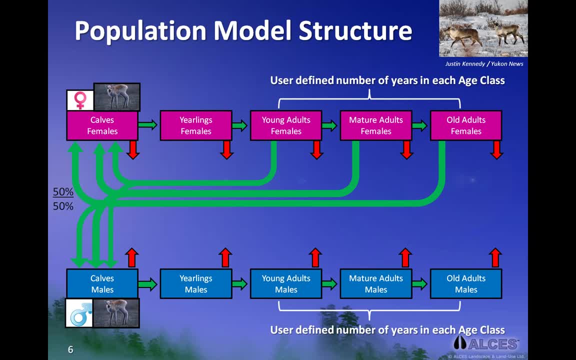 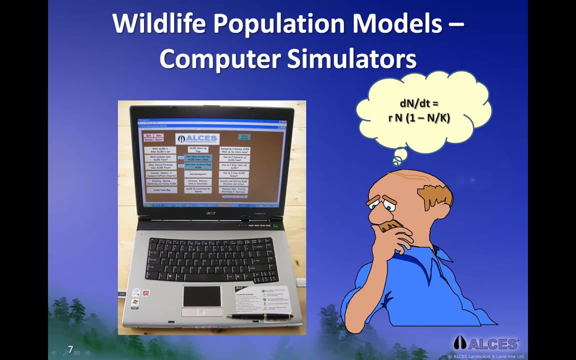 In this example, we also have to specify what we mean by young, mature and old adults and define the number of years within each age class. A key point to take away is that wildlife population models can be quite simple and straightforward and easy to understand. 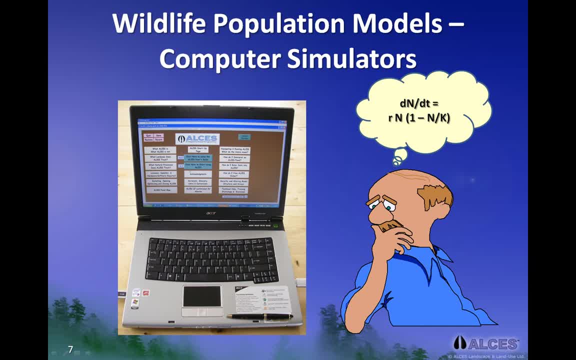 A challenge is that, as we add more details to the models and turn them into working simulation models, the only way we can do the hundreds and sometimes thousands of calculations needed is to use a computer. So we should think of computer simulation models with this in mind. 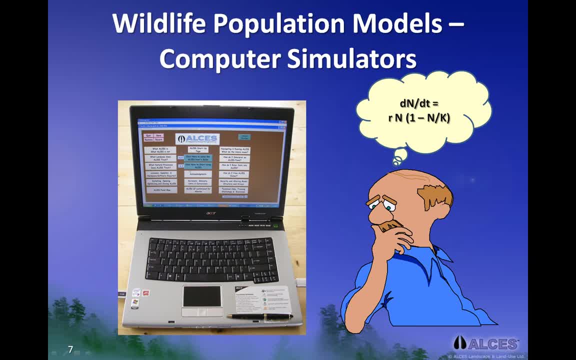 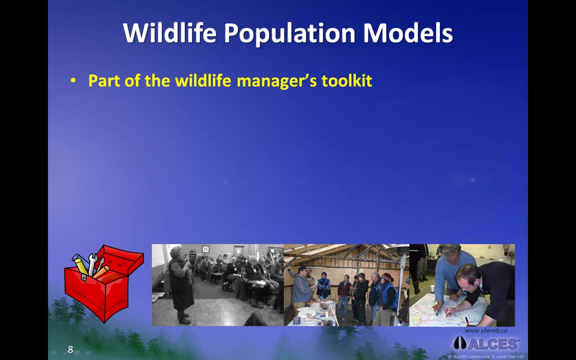 that they are tools that help us visualize and represent the thinking we already do. Indeed, wildlife population models are part of the Wildlife Manager's Toolkit. Models provide a way for management partners, local experts and biologists to communicate, work together and use what they know. 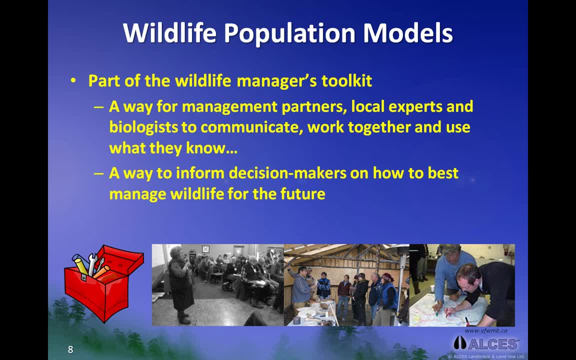 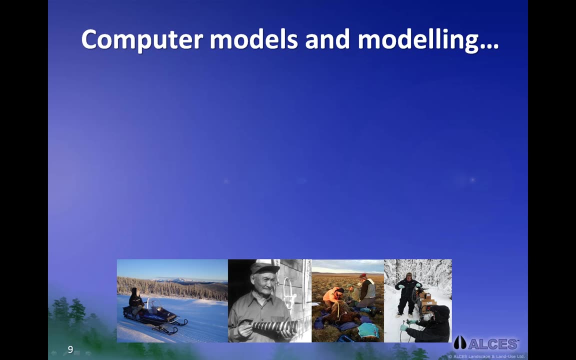 Models may also provide a way to inform decision makers about various options and how to best manage wildlife for the future. In summary, there are three main points to consider about computer models and modeling. Firstly, models and modeling can be used to explain and share our understanding of wildlife population dynamics.